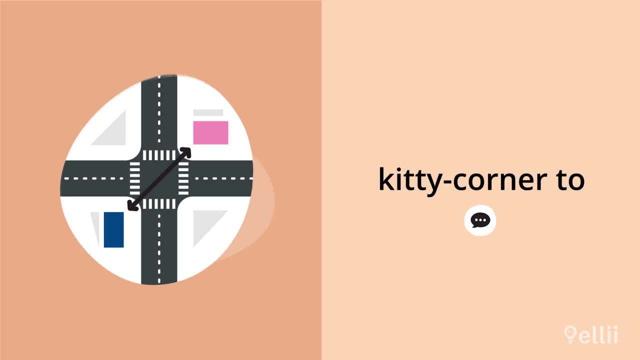 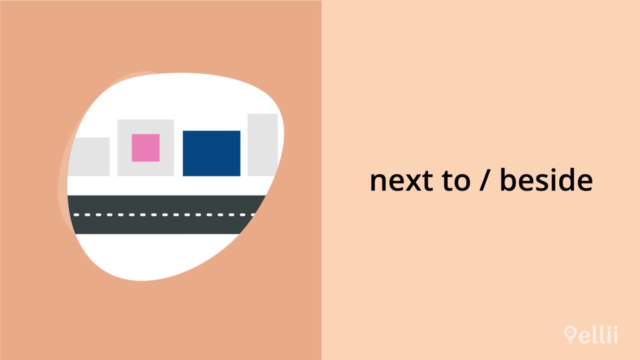 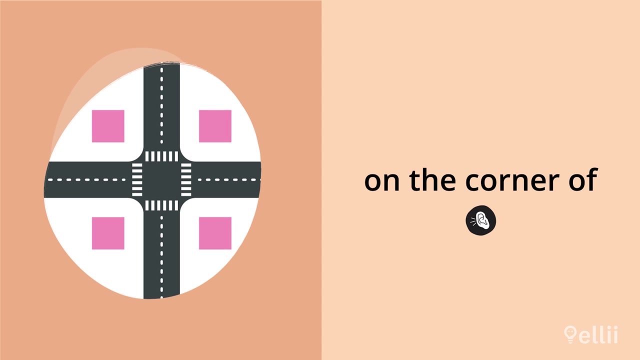 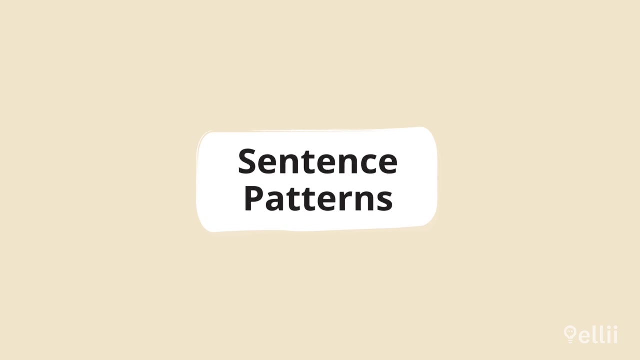 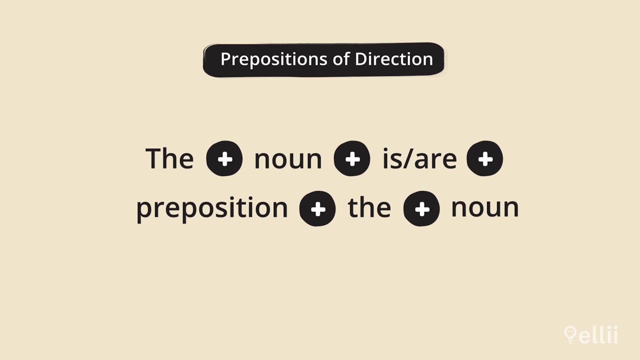 Kitty corner. to Near, Next to or beside, Beside, On, Next, On the corner of The most common sentence pattern for prepositions of direction is the plus noun, plus is, or are plus preposition, plus the plus noun. For example, the shopping mall is far from the bakery. 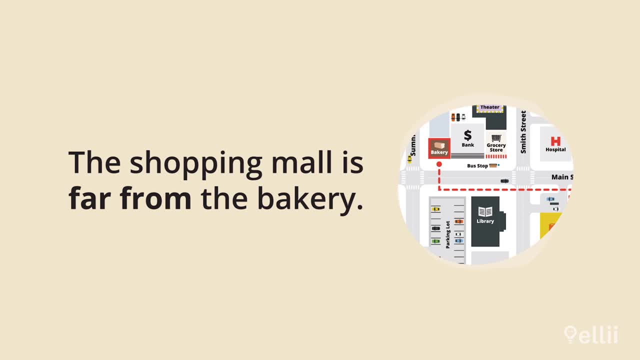 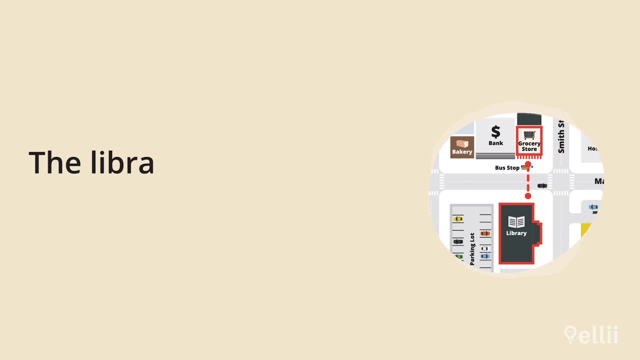 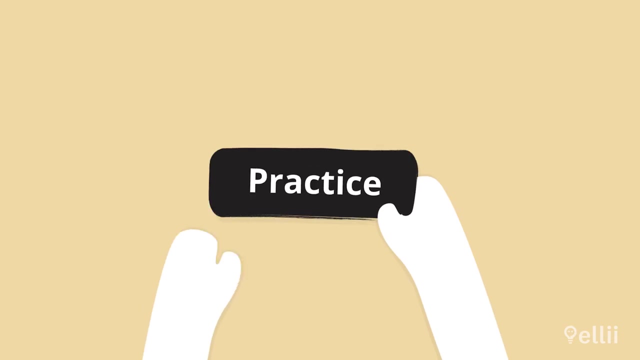 The shopping mall is far from the bakery. The library is across from the grocery store. Guys station is next to the shopping mall. The red car is parked behind the bank. The bank And the grocery store are on Main Street. Uh huh. 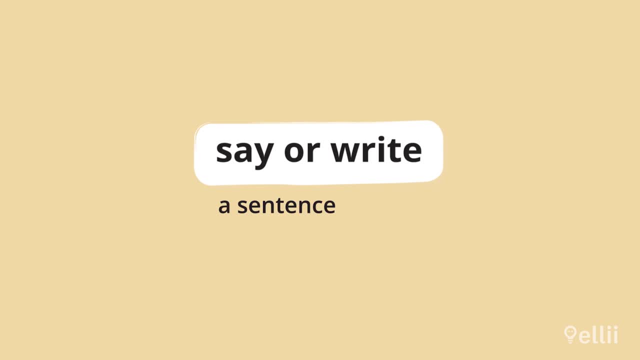 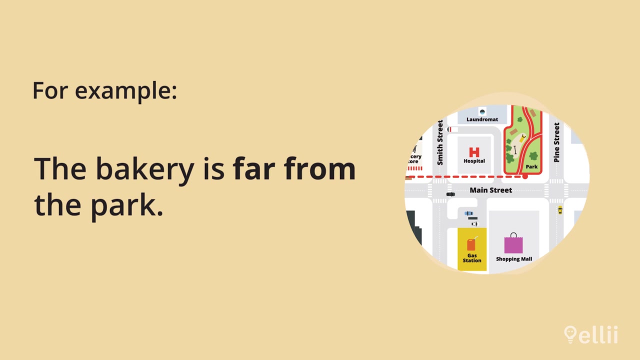 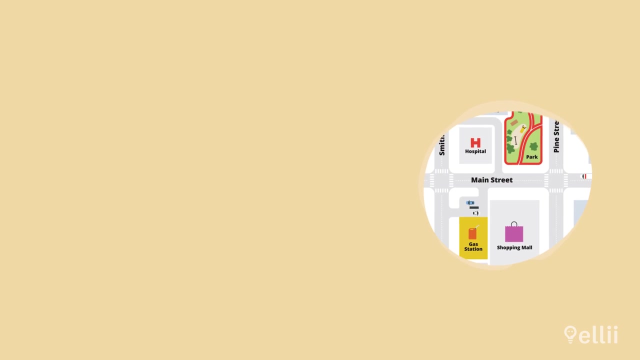 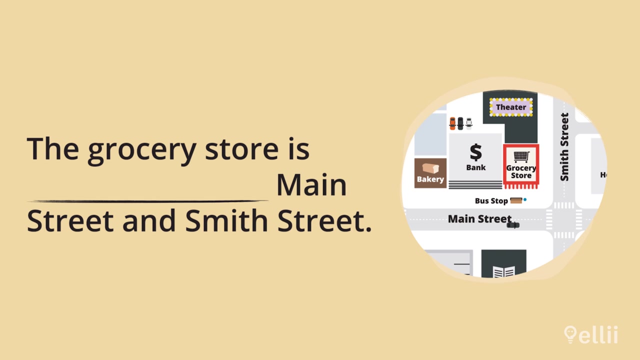 Look at the picture and say or write a sentence using a preposition of direction. For example, the bakery is far from the park. Now you try, The park is across from the shopping mall. The grocery store is on the corner of Main Street and Smith Street. 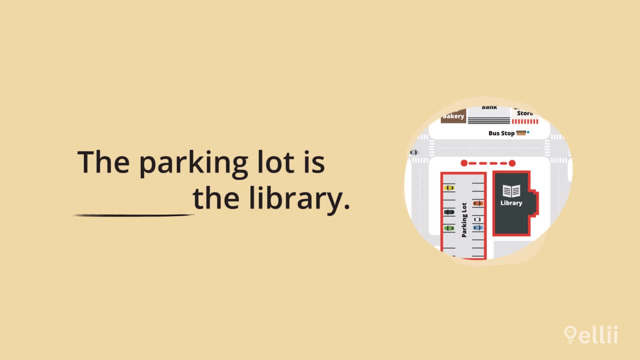 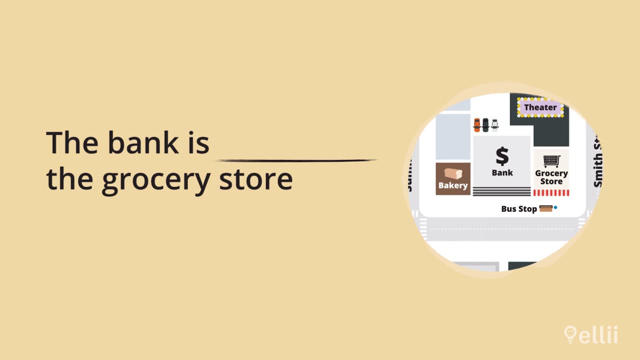 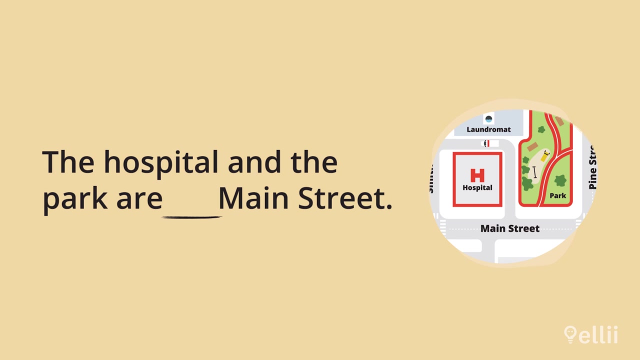 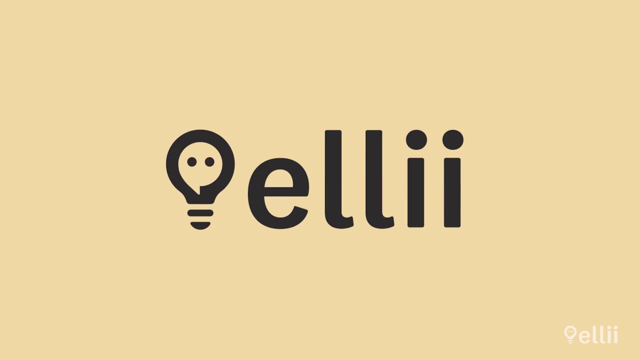 The parking lot is next to the library, The bank is between the grocery store and the bakery, The hospital and the park are on Main Street. Thanks for watching.